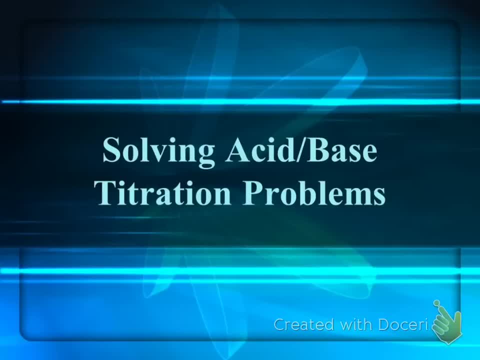 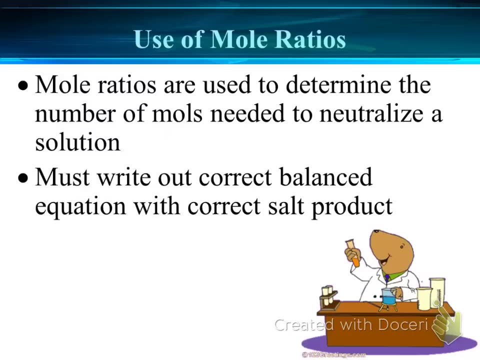 We're going to work on solving acid-base titration problems. To begin with, we review the mole ratio. Mole ratios are going to be used to determine the number of moles needed to neutralize a solution. Neutralization is the key word here. So when we combine an acid, 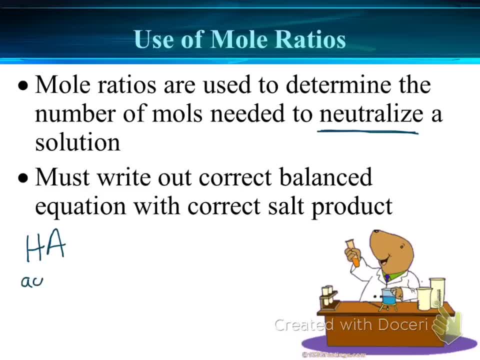 which has the generalized formula of HA. so we can say: this is our acid with a base with a generalized formula of BOH. here's a base, an acid plus a base, combined together to create a salt, where the cation came from the base, the anion came from the acid, salt plus water. 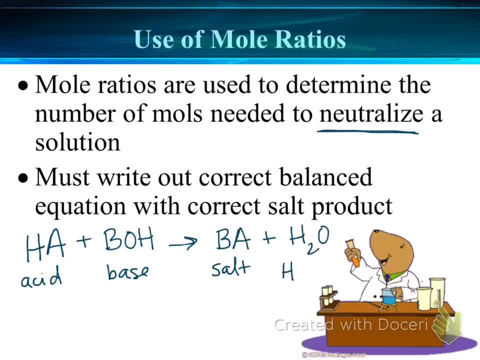 Well, where did the water come from? The water came from hydrogen and hydroxide reacting together. So what's important is that we have hydrogen ions coming off of the acid and the acid donates the hydrogen ions, Hydroxide ions coming off of the base, And when those 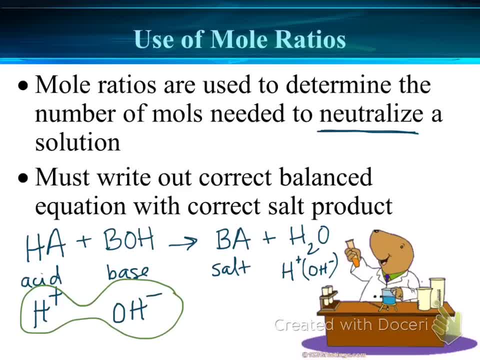 species get together, we make water, And when we've neutralized all of the hydrogen ions with all the hydroxide ions necessary to create water and not have any extra hydrogens or hydroxides, we're done. This is what we're going to be solving for in the titration problem. 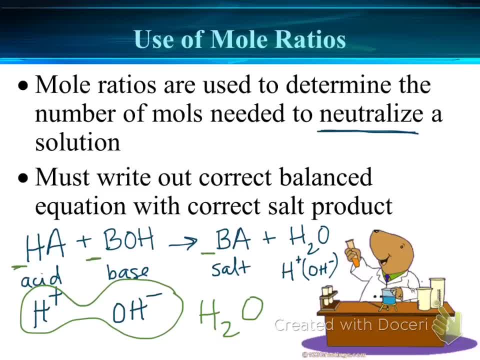 But these ratios are going to be really important. They're going to be really important for us in figuring out how many hydrogens do we need, how many hydroxides do we need. So the ratios are going to be important, So we need a correct. 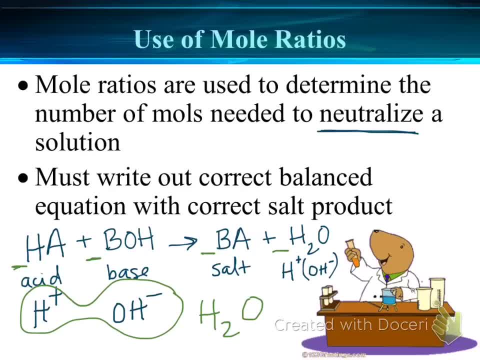 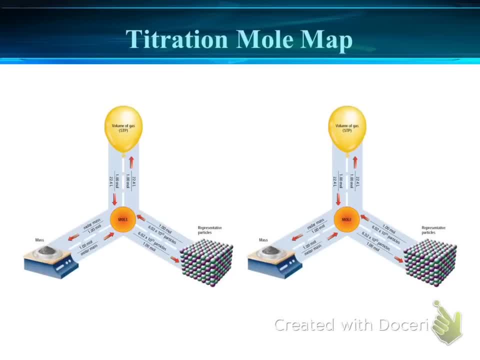 balanced equation with the correct salt product in order to solve the problem. Additionally, we're going to go back to using the mole map. So in the mole map that we started with at the beginning of the year, we had three arms: volume of a gas mass representative. 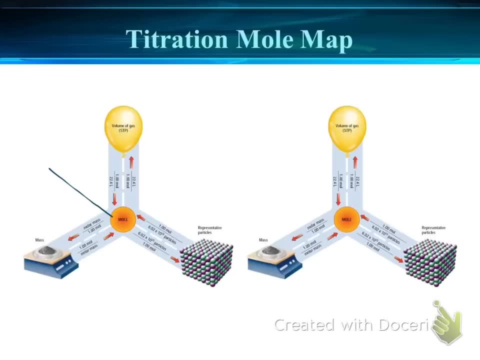 particles, And we added into this an extension for molarity or a mole map, And we added into this an extension for concentration And we said that molarity is equal to moles of solute over liters of solution. So I'm going to add molarity to both sides of my 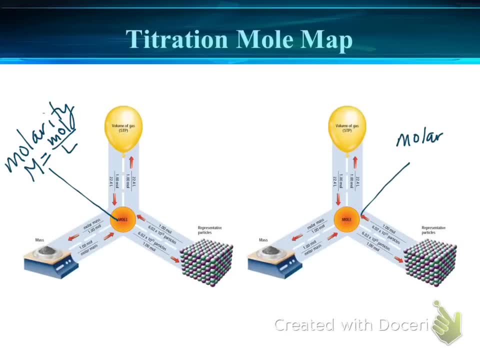 mole map here. So we may not necessarily be solving for molarity, but if we're working with concentrations we want to use this molarity equation And we said we could connect the double mole map by using the mole ratios from the balanced chemical equation. So when we 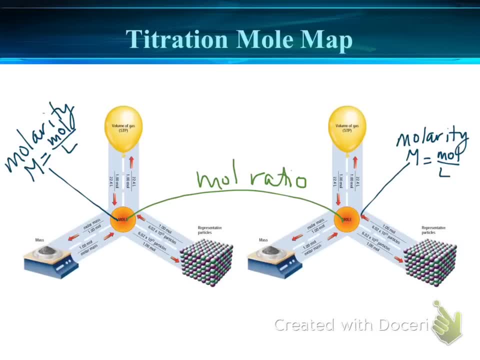 solve problems involving acid-based titrations. we're typically going to start out right over here. So we're going to start out with a known amount of a known concentration. Then we're going to have to go through several steps. We start with what we know We'll use. 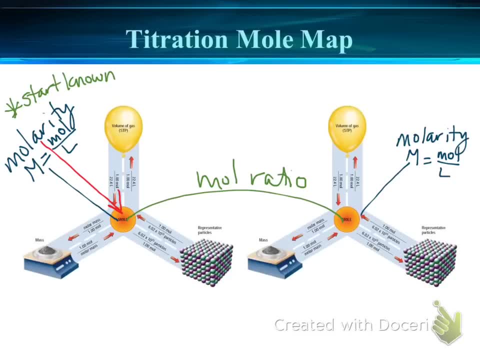 the molarity equation in some form to get us to moles. Then we'll go from moles of our known to moles of our unknown, Using the mole ratio, And then we'll go from moles of our unknown to molarity or volume. 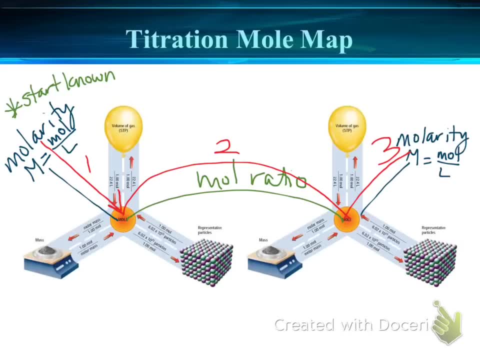 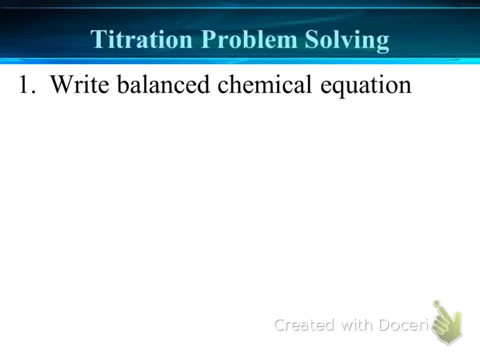 in the next step. So three major steps. They all stem off of the first step, which is actually the balanced chemical equation. Now, typically this is the hardest part for students, So you want to make sure that you remember when you're balancing chemical equations, you first 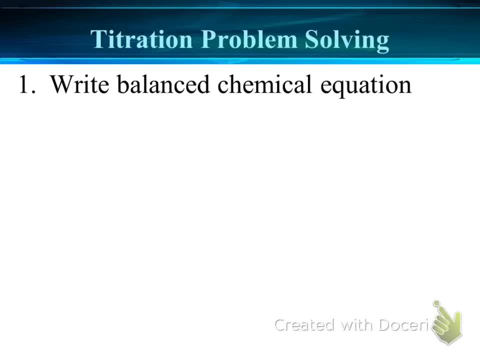 have to balance each individual substance, your reactants and your product species. So don't forget to look for charges and have your chemical equations balanced. And then have you written the right subscripts, And is the subscript supposed to be there? Once you have the balanced chemical equation, we're going to follow the mole map to help us out. 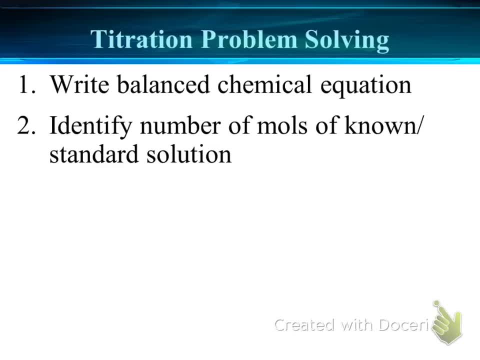 We'll first identify the number of moles of known in our standard solution, And since we're typically going to be working with molarity, we know that molarity equals moles over volume. So what we want to do is rearrange this, And we know that moles will be equal to molarity. 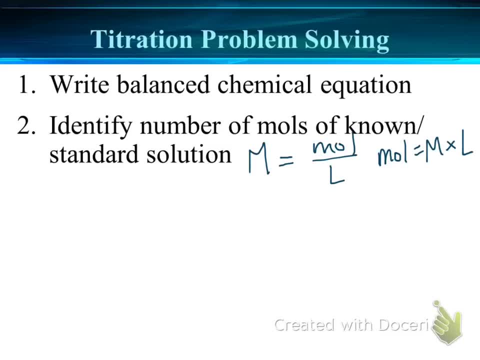 times volume, Okay, molarity times liters. Next step is going to be to convert to moles of our unknown using the mole ratio, And then, finally, we'll solve for our unknown. And when I say that we're going to solve for our unknown, 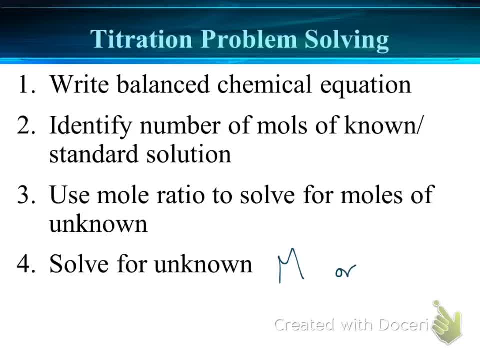 we could be solving for molarity, or we could solve for volume. We could solve for liters. Once again, molarity equals moles over liters. If I'm solving for liters, then liters will be equal to moles over molarity. Okay, 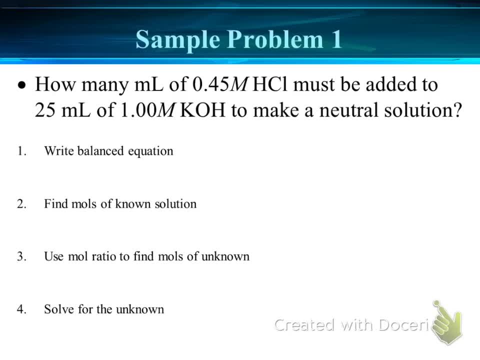 We're going to be able to rearrange the equations important. So let's take a look at a sample problem. Here we go. How many milliliters of 0.45 molar hydrochloric acid must be added to 25 milliliters of 1 molar potassium hydroxide to make a neutral solution? So step number: 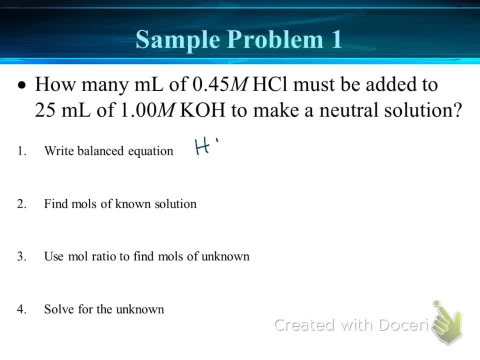 one is write the balanced equation Hydrochloric acid plus potassium hydroxide. All right, Rearrange, We're going to form a salt-potassium chloride, Potassium chloride and water, H2O. Okay, I can look and see that I have one potassium. 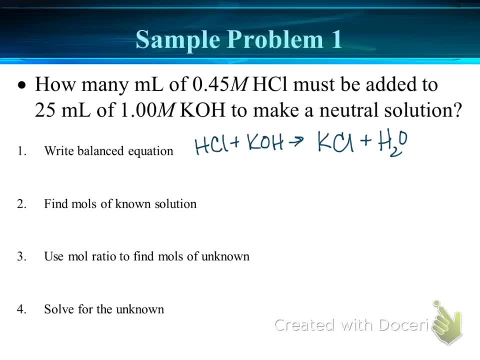 on each side, one chlorine on each side, two hydrogens on each side, one hydroxide on each side. So this one's nice and balanced. Now, when we did our stoichiometry problems earlier in the year, I said to use the equation to help you organize the information. So let's. 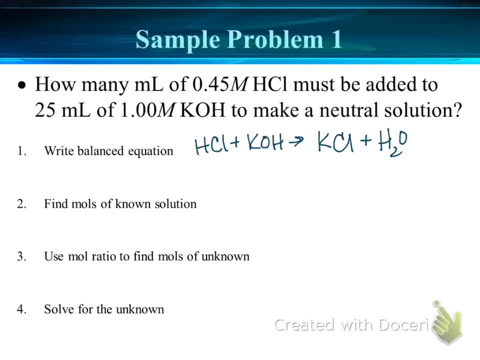 do that again. So underneath hydrochloric acid, I am going to write the concentration, which is 0.45 molar. Okay, And I don't know what volume. That's what I'm trying to solve for. Okay, Under potassium. 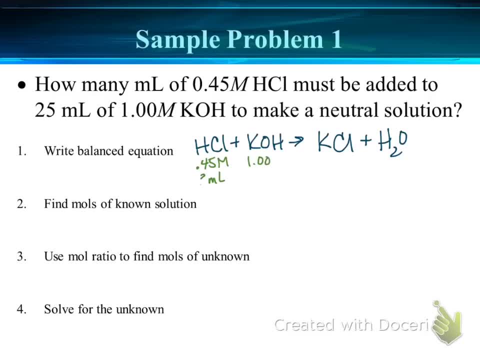 hydroxide, I'd have a 1 molar solution and I have 25 milliliters. So this allows me to see all of the information in simple format. So now I can get into solving the mathematics, the stoichiometry, the titration kind of stoichiometry for this problem. So first I want to find moles. 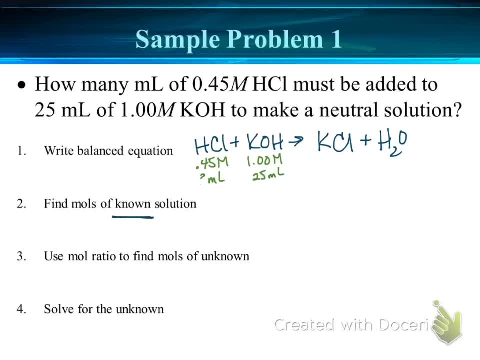 of my known solution. Well, what is my known solution? My known solution is what I know the most about. So in this case, I know the most about potassium hydroxide. So that's going to be my known solution. Okay, Reviewing once again, If molarity equals to moles over. 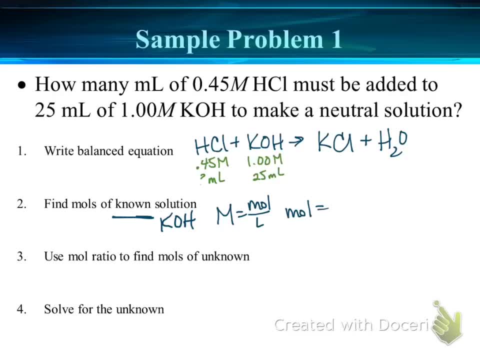 volume, then moles is equal to molarity times volume. So that's what I'm going to do here, Right? Okay, So I've got 0.25 molar times 0.025 liters. Okay, Remember, we want to use liters, So 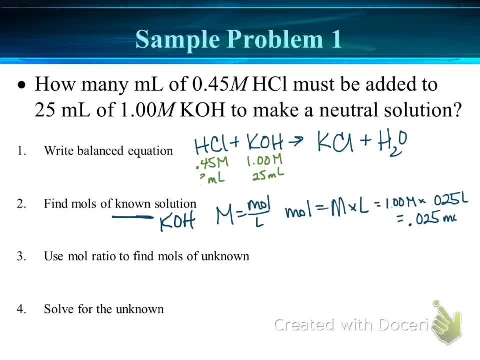 that gives me 0.025 moles of my potassium hydroxide solution. Okay, So I found moles of my known. Now I'm going to use the mole ratio to find moles of the unknown. So this time I have 0.25. Oops, Sorry about that. 0.025 moles of my known. 0.025 moles of my known. Okay, Now I'm going to use the mole ratio to find moles of the unknown. So this time I have 0.25.. Sorry about that. 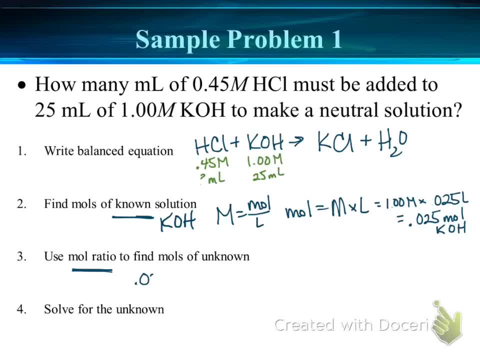 I have 0.025 moles of potassium hydroxide. My mole ratio is 1 to 1, but let's write it out for ourselves, because not every problem is going to be 1 to 1.. So get in the habit. 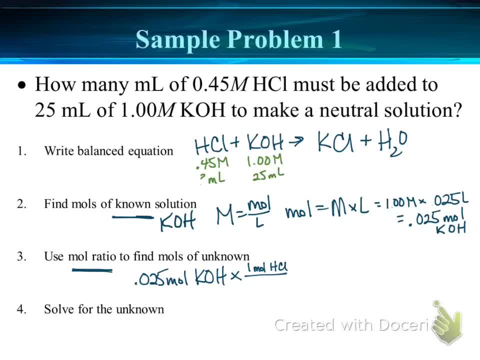 of doing this now. Moles of what I'm going to on top, moles of what I'm going to on the bottom, And remember, the ones come from the balanced chemical equation, And so this time I know that I still have 0.025 moles. 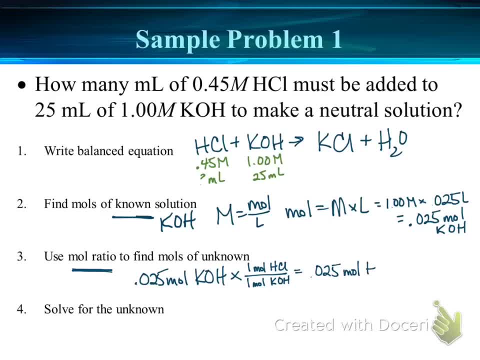 0.025 moles of potassium hydroxide. 0.025 moles of HCl. HCl is my unknown. My unknown is HCl. That's what I'm trying to solve for And this particular problem I'm being asked to solve for volume. Once again, 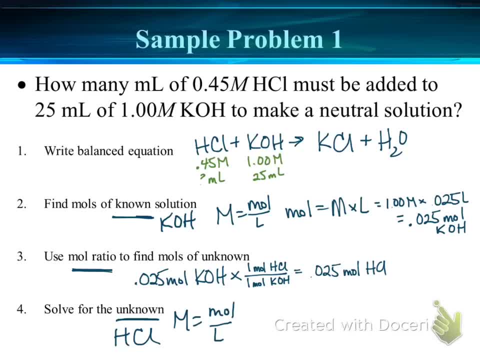 if molarity equals moles over liters. rearranging this equation, I get liters or volume equals moles over molarity. 0.025 moles of HCl. 0.025 moles of potassium hydroxide. 0.025 moles of potassium hydroxide. 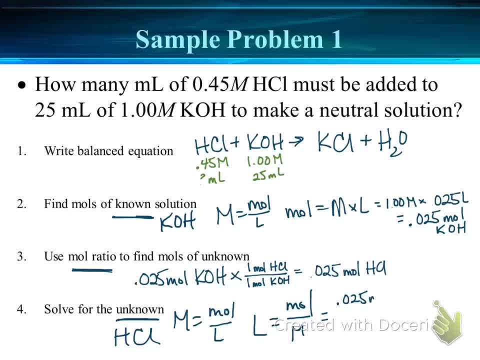 0.025 moles of potassium hydroxide. 0.025 moles of HCl. 0.45 molar is the concentration. the problem gave me Solving this. I get an answer of 0.056 liters, And if you move the decimal one, two, three places, then you: 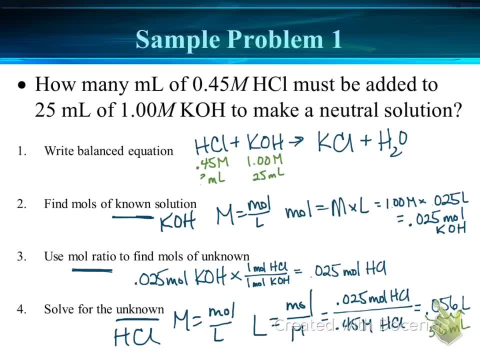 get the answer of 56 milliliters. So take a moment to look at all of those steps. We started with the balanced chemical equation Check We found moles of the known solution. Check We used the mole ratio to find moles of the unknown. Check 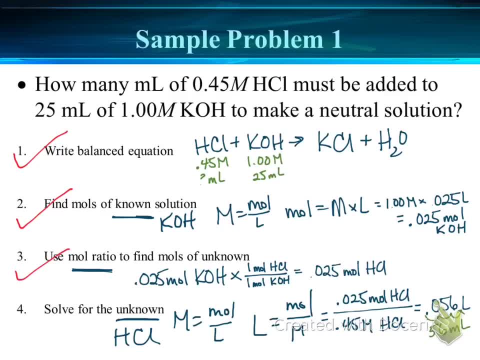 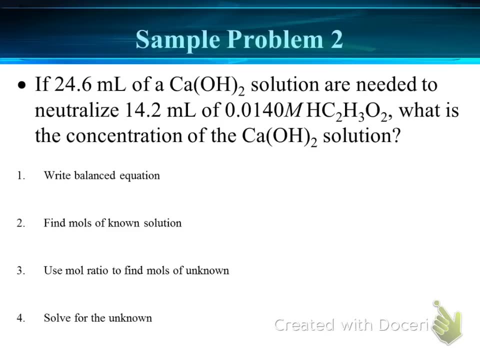 And then we solved for the unknown, and in this case we were solving for volume. So let's see another problem, This problem we're being asked to solve for concentration. Notice, the steps are exactly the same. We'll just have a rearrange order Check. 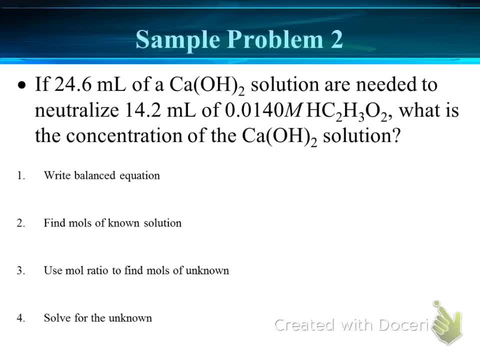 You were asking me to use this greater than value formula to solve for concentration. We've got aшая. Now check thisrist dock: 0.05 assembled ground, Yeah, 10.. You can see this ошиб quieter: 0.25 LN .015 equal to 32.. 7.. 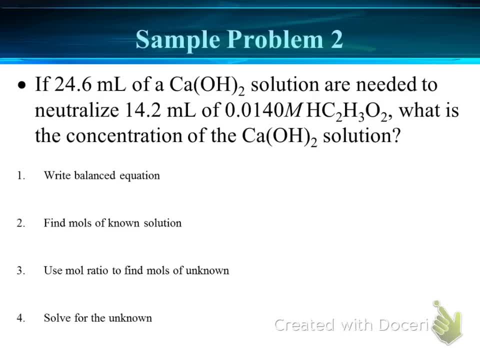 All of this example you just did here and wow, 0.221 moles out, A impact: 0.21鉄. total: 0.10. foritute rearrangement of the molarity equation into number four, which is actually a little bit easier. 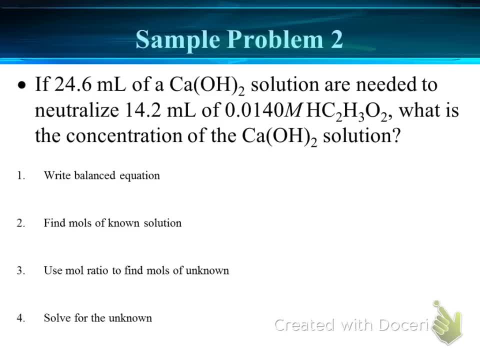 because we're solving for molarity and not volume this time. So once again, start with the balanced chemical equation. You've got a lot of different species to deal with here, so it can be challenging. Calcium hydroxide, CaOH2, plus acetic acid, HC2, H3O2,. 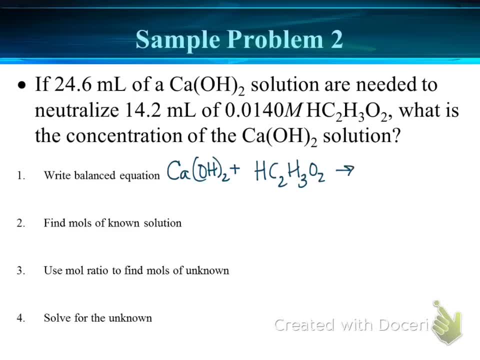 goes to our salt, calcium acetate, balanced for all of the species and water Going back through and balancing them. Sorry about that. I'm going to need two acetates And I'm going to need two acetates And I'm going to need two acetates. 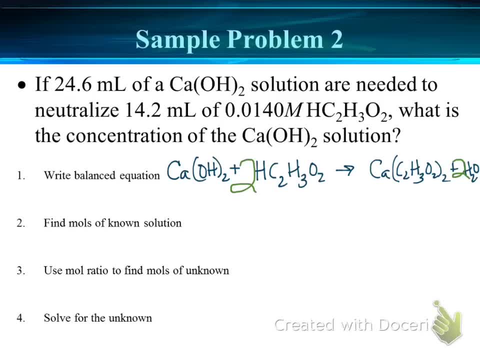 And I'm going to need two acetates, need two waters, So balanced chemical equation. Once again, organize the information that was given to you in the problem. So if I take a look at the problem, I am told I have 24.6 milliliters. 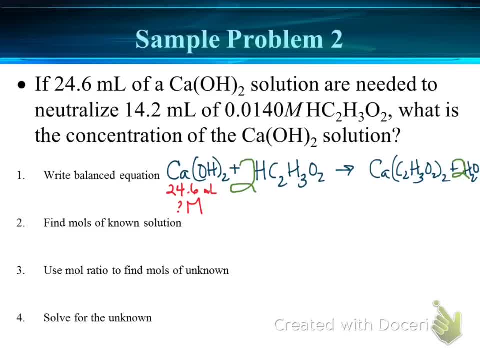 and I want to find molarity, And then I have 14.2 milliliters and then known molarity already. So remember, the moles of known solution is the one that you know the most information about. So I know the most information about acetic acid. So for acetic acid I'm going to find moles of my known 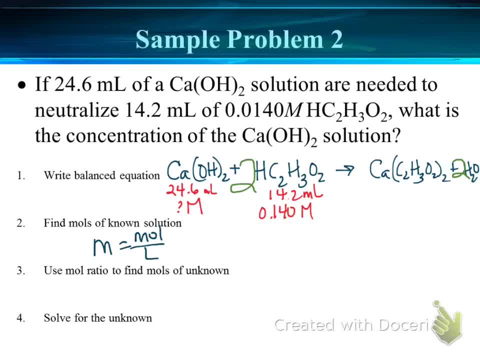 So molarity equals moles over liters. So moles equals molarity times liters. In this case I have 0.0140 molar times times 0.0142 liters. Remember I've converted liters to liters and I get a complicated looking. 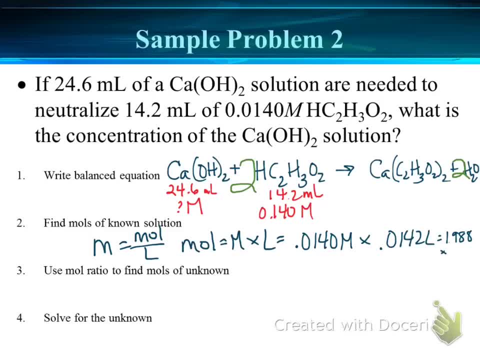 number: 1.988 times 10 to the minus. fourth moles: Very, very small number of moles. Now I'm going to use the mole ratio to find moles of my unknown: 1.988 times 10 to the minus. 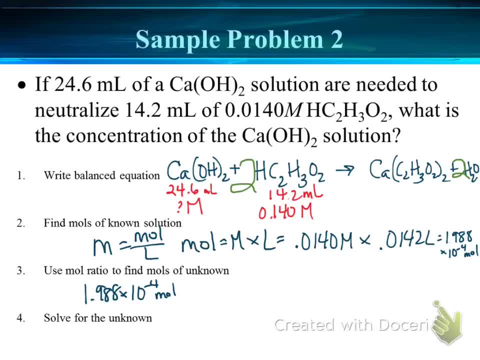 fourth moles. This is of the acetic acid right, So H2, H, H, C2, H3O2.. You can tell I'm in my classroom doing this One mole of my unknown, which is what I'm solving. 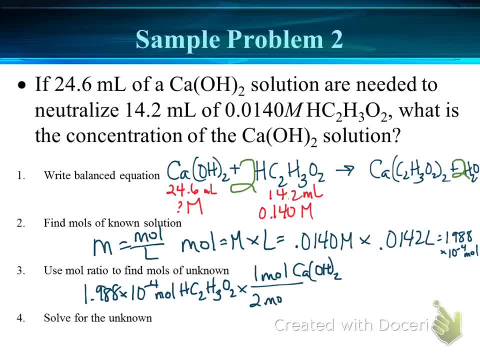 for On top two moles from the balanced chemical equation of acetic acid And I get 9.94 times 10 to the minus fifth moles of my calcium hydroxide. Now I want to solve for the unknown In this problem. I want to know moles. Moles is just. I want molarity, Molarity is just. 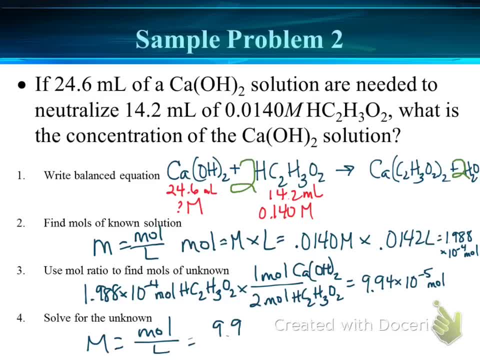 moles over volume. So I have moles. Volume comes all the way from up here, So I've got to convert that into volume in liters, so 0.0246 liters. And then my molarity- here is a small molarity: 4.04 times 10 to the minus third molar. 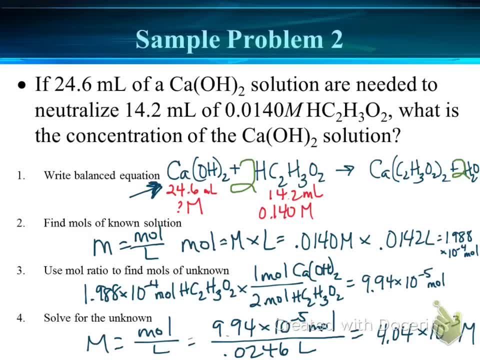 So I know that's a lot of information to look through, but you've seen this before. We've done these type of problems before using the double mole map. It's just using the molarity component as part of the double mole map. Write a balanced chemical equation, Whichever one you know, the